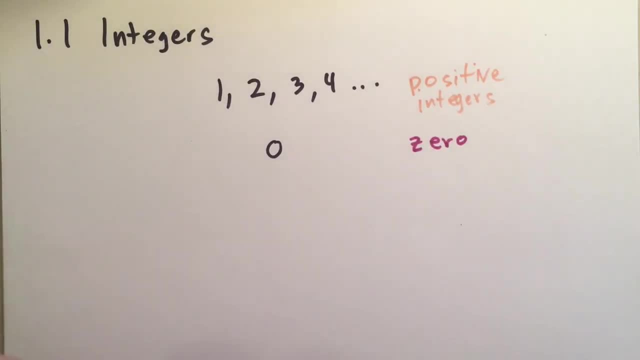 that zero was. But this is a very special number. It's a very important and significant number. It's going to show up again and again as we learn math. It has some very special properties. All right Now to understand these numbers. his example in the book is hilarious. He says: 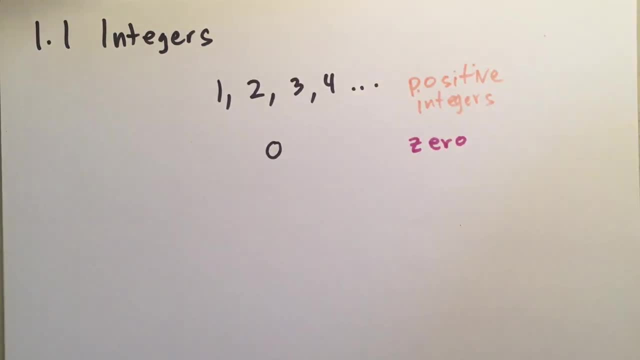 these numbers could represent the score you get on a test in math. If you got 100,, that means you got all the answers correct. If you got 1,, that means you only got one of the answers correct. But if you got a zero, that means you got nothing right and you don't. 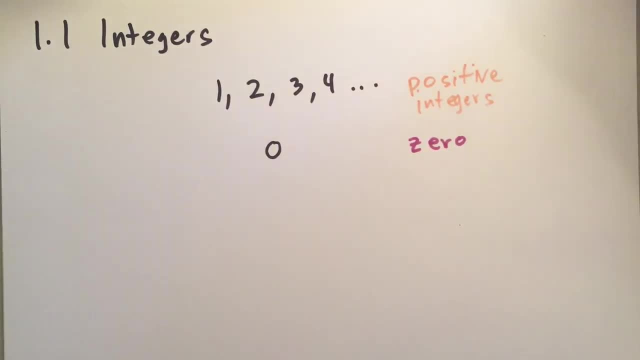 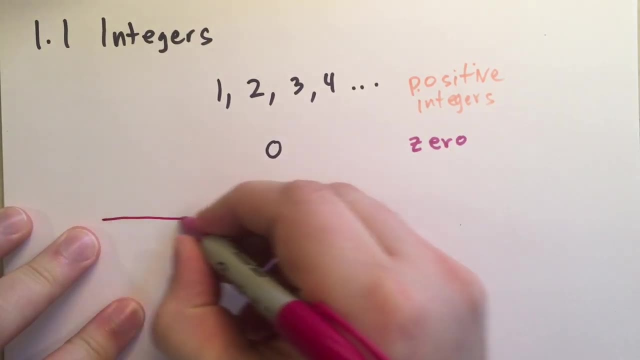 know anything about math. But hey, we're here to learn, right, So we can represent these numbers as if they're on a line, So we can draw a line And then on this line we choose some arbitrary point to be our zero. 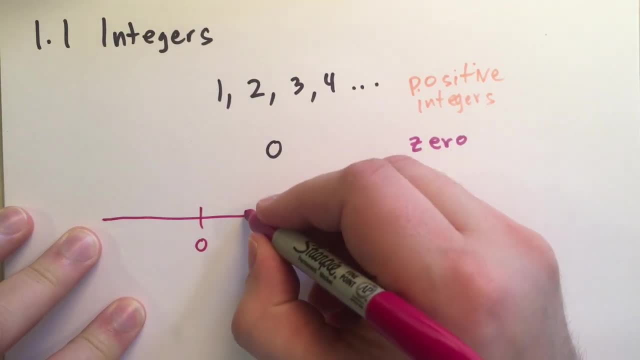 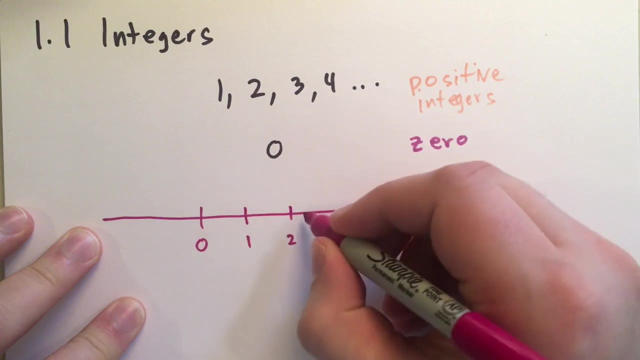 I'm going to choose this point to be zero. And then we stretch out a unit distance- It doesn't matter how long it is- And we call that 1., And then two of those distances we call 2., And three of those distances we're going to call 3.. 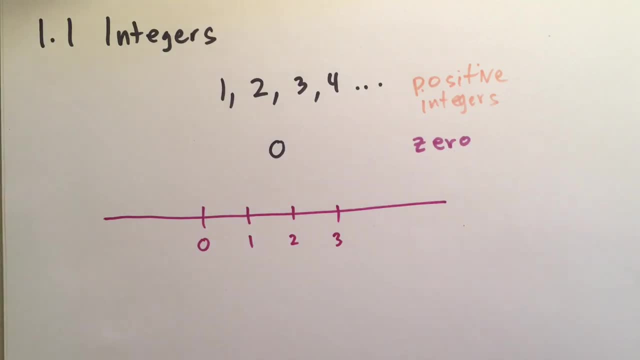 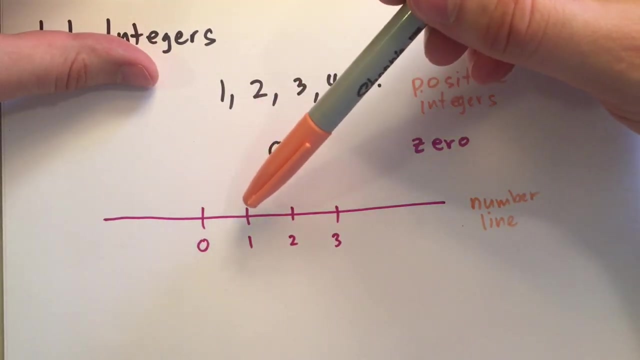 And this number line is an important concept. It's a really great way to visualize and understand what the numbers are. Let's use this peach color here. that's called the number line. But one thing I want you to think about is that the number line isn't really representing. 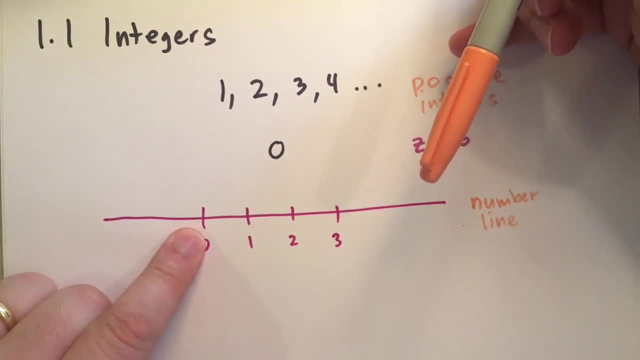 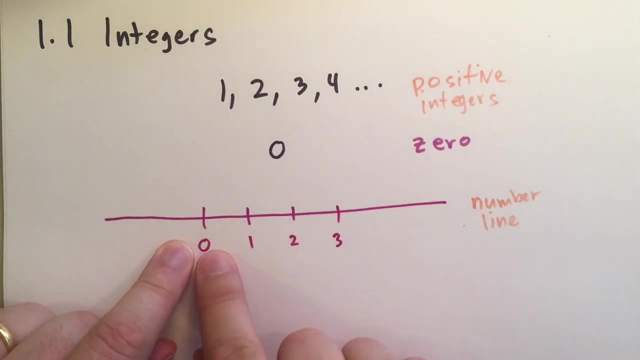 positions in space, aside from where the zero is. The zero tells you that on this spot on this piece of paper, this number line begins. These numbers tell you a distance from that position. So 3 really says you've gone three units to the right And you can see there's. 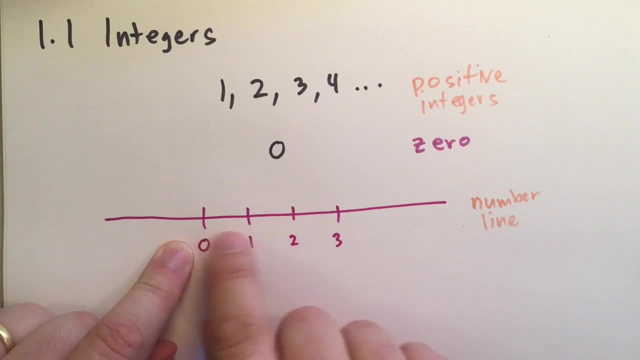 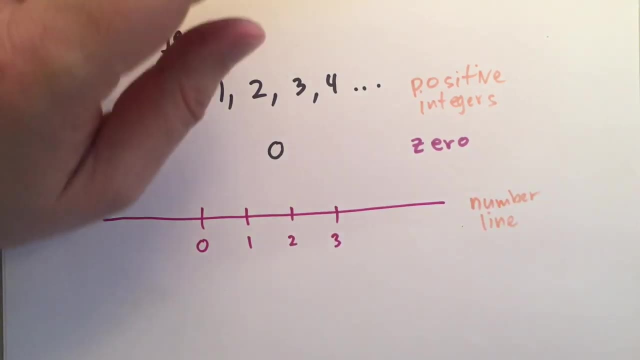 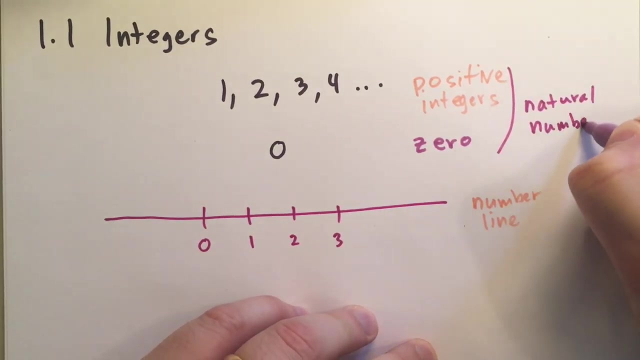 one, two, three units in between here, and three And 2 says you've gone two units to the right, The zero and the positive numbers together. we call these the natural numbers. Why we call them that? Because they arise naturally a lot. Don't get too concerned about the names. 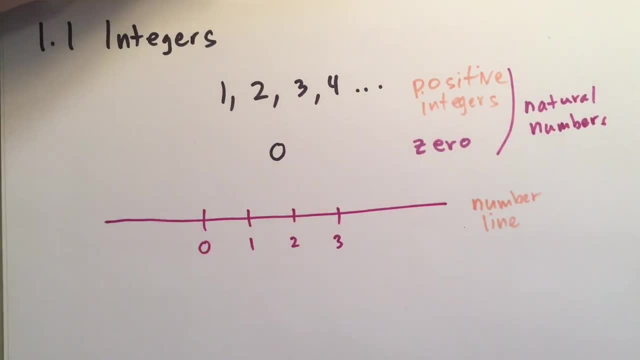 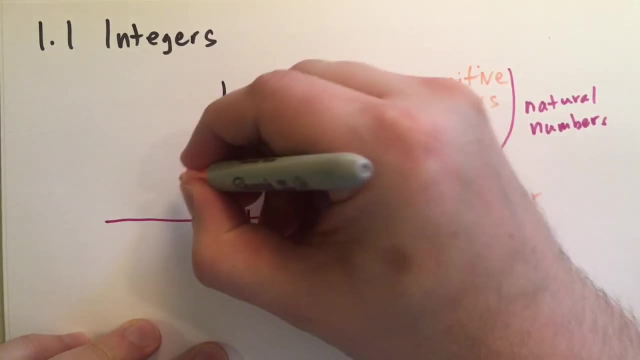 we choose for things, It's not terribly important. We just give them names to make sure that they're different And we know what we're talking about when we talk to each other. This special point here where the zero is. we call that the origin We'll be talking. 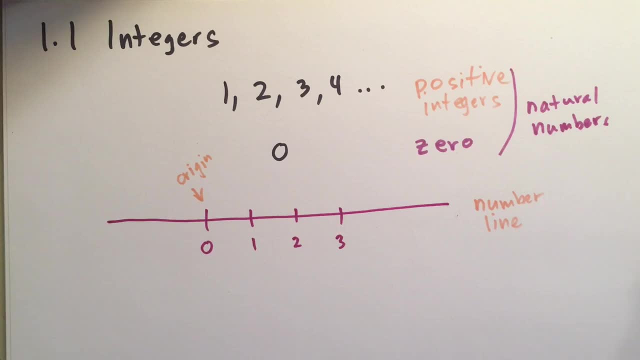 about the origin a lot all throughout. math And the natural numbers can be used to measure other things he says in the book. For example, a thermometer- You can use a natural numbers to represent how hot it is outside. If you're in Celsius land, 0° would be freezing and 100° would be, the Earth is boiling. But if 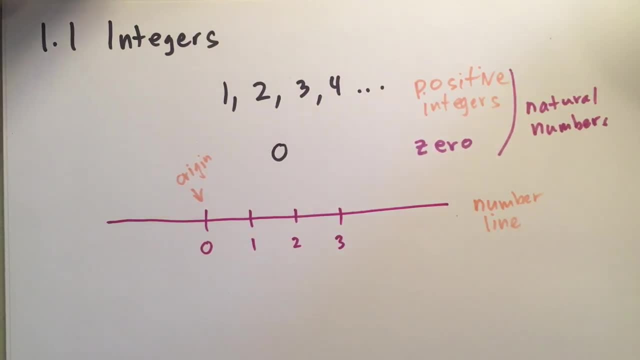 you're in Fahrenheit land- 0° would be below freezing, well below freezing, And 100° would be a very warm day, a hot day. So that means that these numbers- it depends on what you're talking about and how they work- 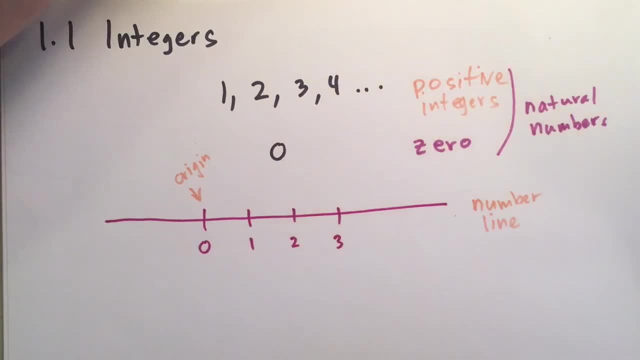 Well, on the thermometer, if it's a very cold day in Celsius land or in Fahrenheit land, then you notice that the thermometer drops. You can go down to a negative one, You go down to negative two. And what does that mean? The negative numbers. 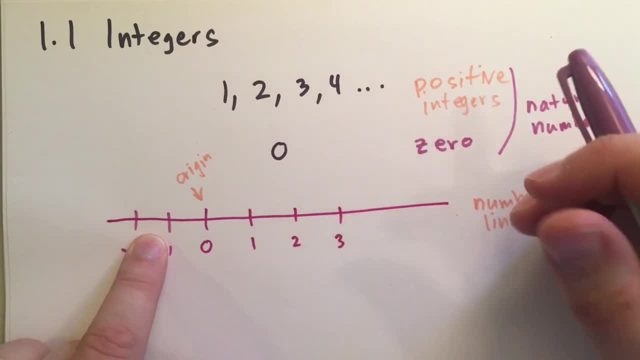 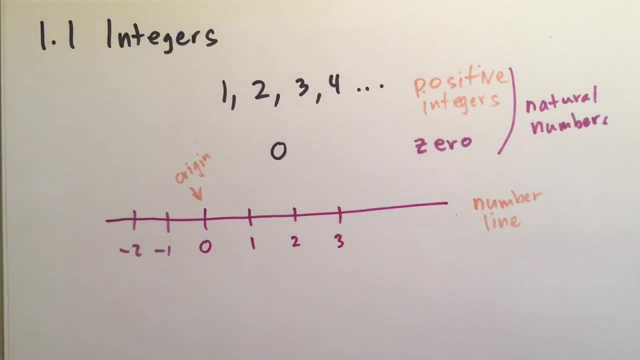 means you're moving that many units to the left. I kind of made that one a little shorter or smaller. It should be the same size as the other ones, And this obviously goes off into negative infinity. And so these numbers- negative one, negative two, negative three, et cetera, we call. 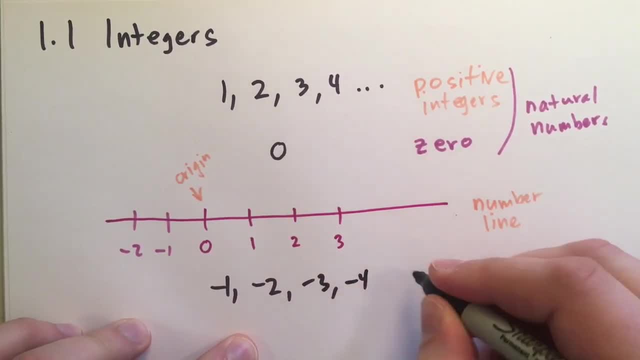 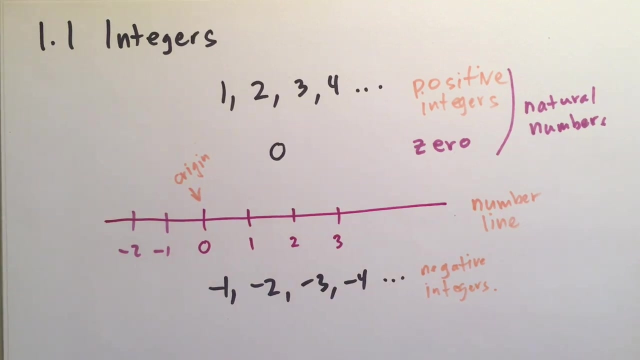 these the negative integers. Let me write that down for you. These are the negative integers. Let me use the pink again, or the peach, the negative. So now you know about negative numbers. That's basically everything you need to know about them. 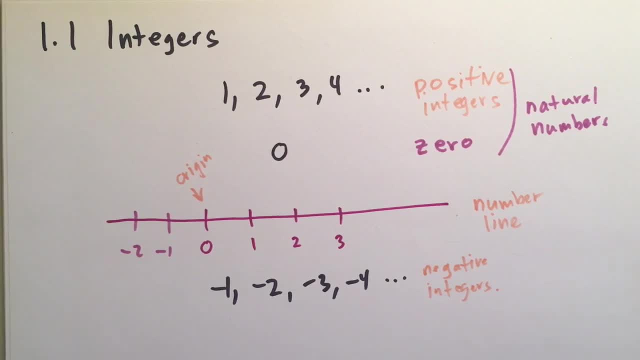 We're going to learn what you can do with them later. This conversation that we're having right now is something that we're going to have again and again in math, where we introduce a new type of number, something that you can do with it, And so we're going to use it, And so we're going to use it, And so we're going. 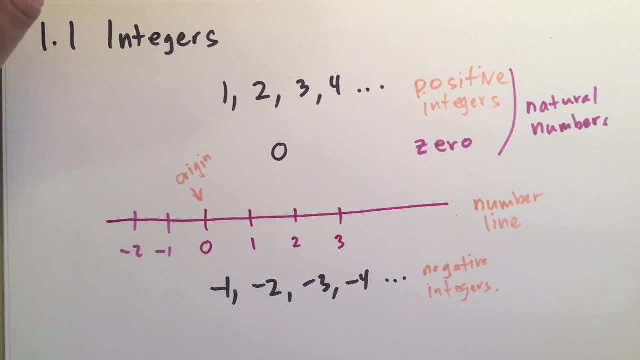 we can do math with. We talk about where it starts, how it moves, how you can go from one number to the other, and then we begin a discussion about the operators we can apply to the numbers. In the case of integers, there's a very important operation you can use. It's called addition. 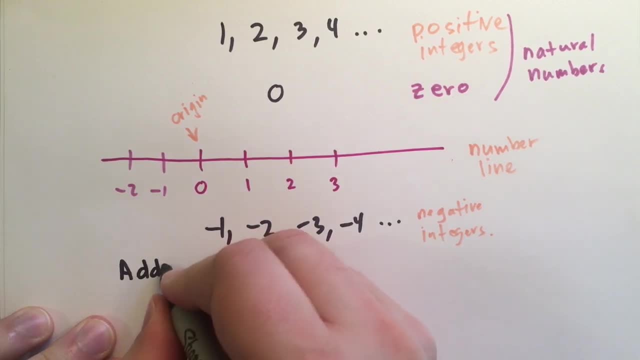 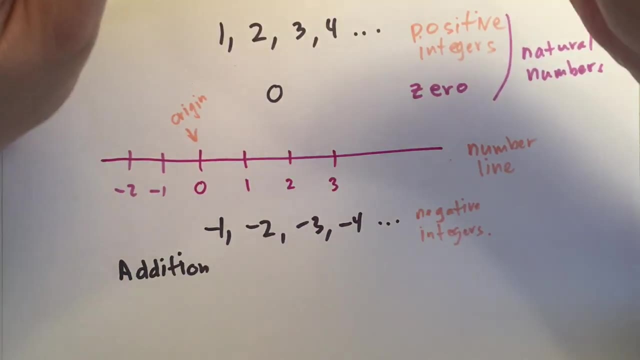 I'll write that in black here, because it's important. You learned about addition at a very young age. If you had two pieces of candy and your friend had two more, then if you took his candy you'd have even more than two. You'd have four. 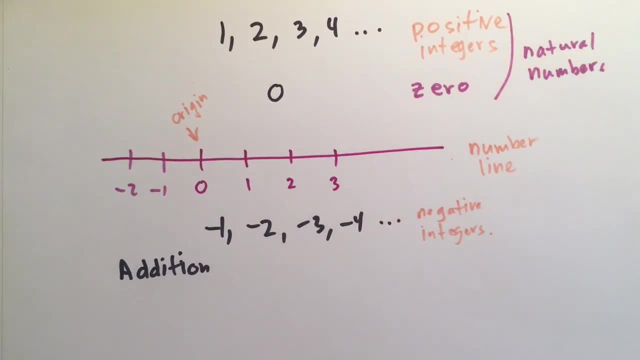 We write down addition like this: We take some integer, we put that little cross sign and we put some other integer, in this case seven, and then we have these two bars here and then we write 12.. Let's analyze what this sentence says. 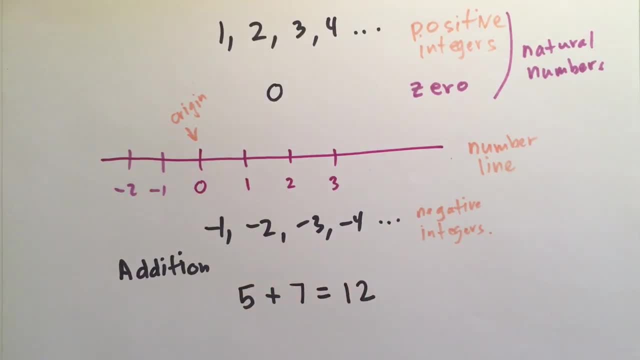 These equations are just sentences. If you go back to the old math papers, you'll see that people actually spelled out in their native language the math sentences. They didn't use symbols. This symbol right here actually comes from a Latin word. that means: and This means add, This means 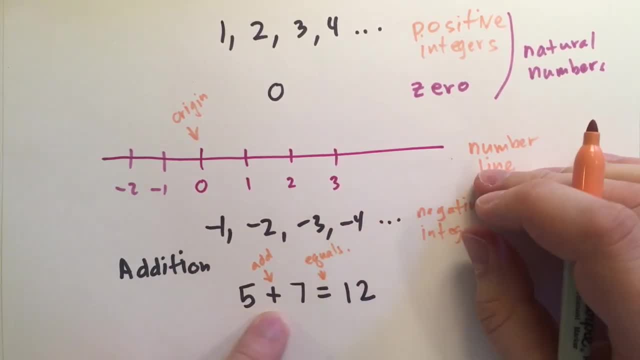 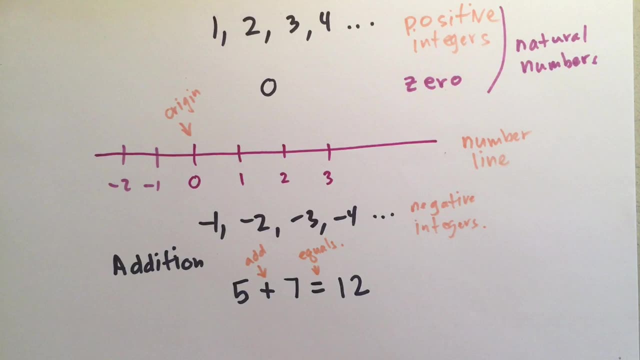 equals Adding says that you're taking this thing on the left and you're taking that thing on the right and you're bringing them together like you would pieces of candy. The equals says that both sides are the same. They're balanced If there's 12 things on this side. 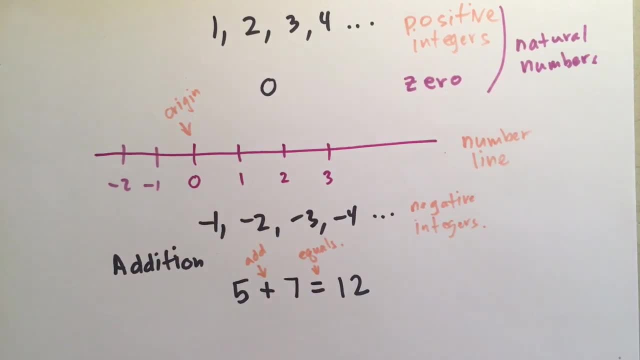 that means there's 12 things on that side and you can switch the equals sign anytime you want. We call this the reflexive property. Things that are equal can be flipped around like that and it doesn't change anything. So 5 plus 7 equals 12, and you learned that in elementary school. 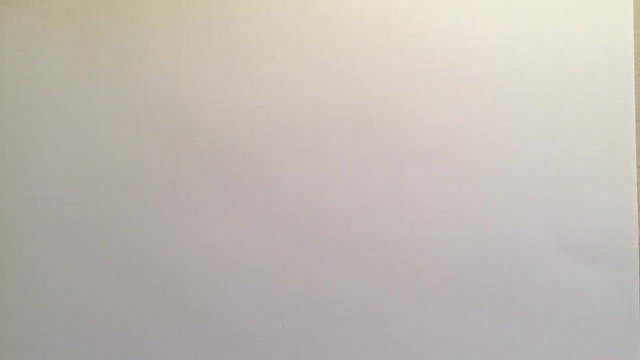 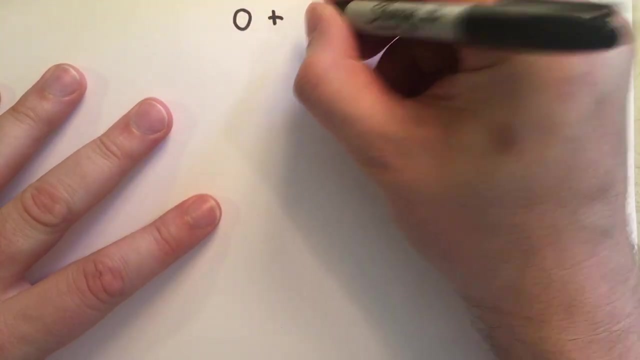 But let's learn some more interesting things about addition. The first interesting thing we're going to learn about addition is that when you take zero and you add any number, and how do you write any number? Well, in this case, I'm going to write the letter A. 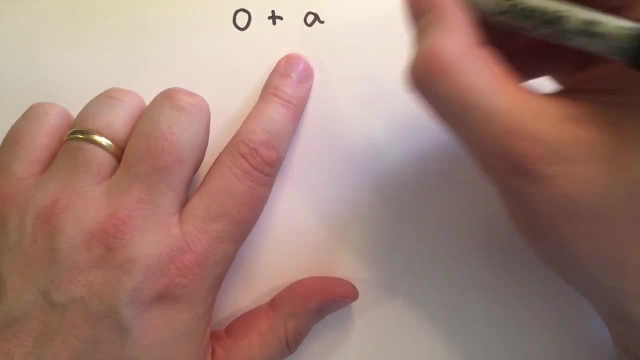 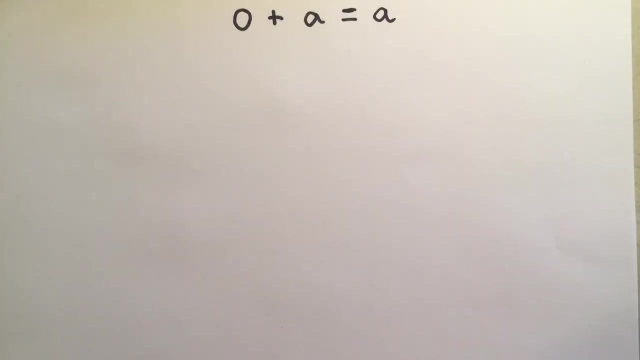 And what this A means is. it could be any number in there And then we're going to write this: equals what? If you take zero and add it to any number, you're going to get that same number back. So this means any number. 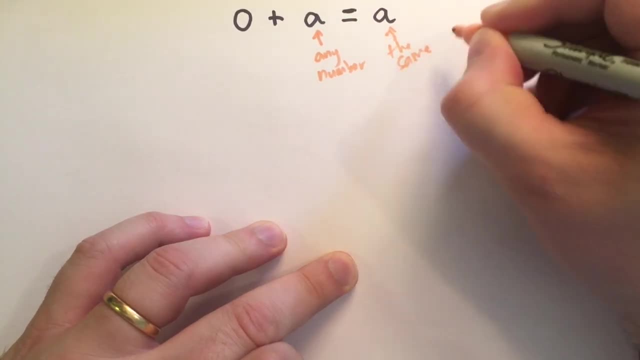 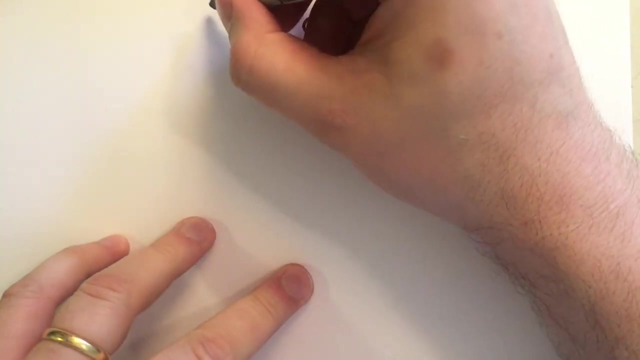 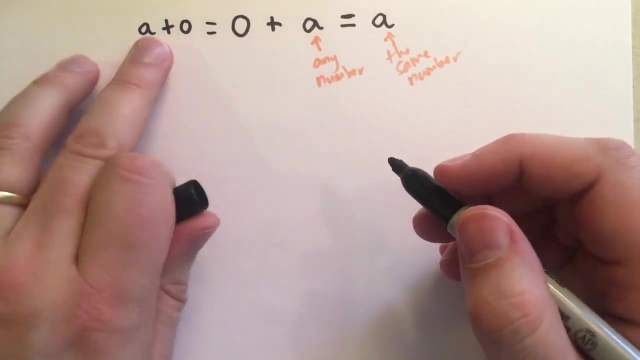 And this means the same number. This is a very important property of addition, And we'll be using this all the time, And we can even write it this way too. We can say: you start with any number and you add zero. It's the same as adding zero to any number, either way. 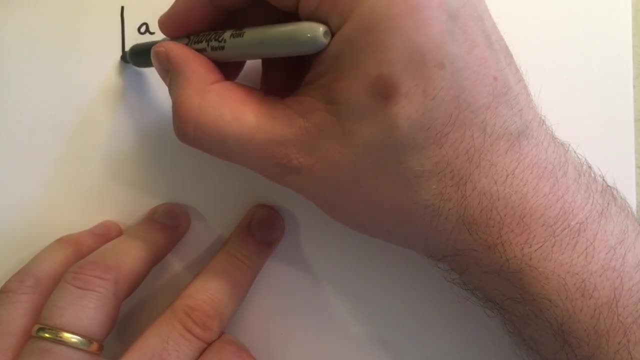 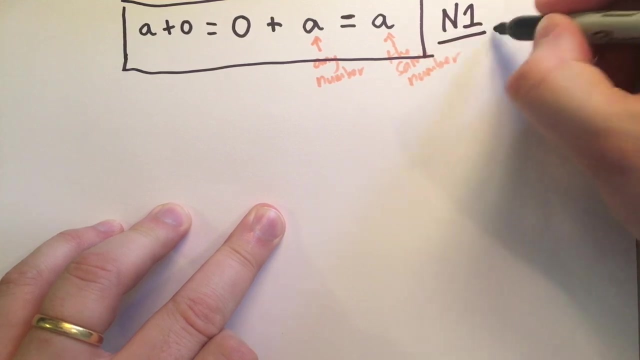 And it's the same as adding or just having that number by itself. I'm going to draw a box around this. Okay, And in the book he labels this equation N1.. Okay, In math textbooks we label our equations and we refer back to them constantly. 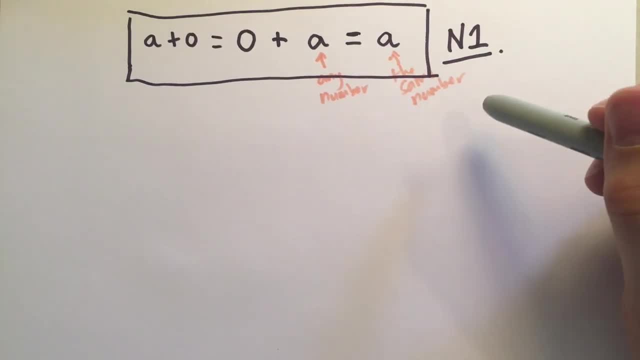 So you have to remember which equation is which, And if you need a flash card or if you just need to be able to jump back to the book book and remember what they're talking about when they say n1,, then you need to do that. So we're. 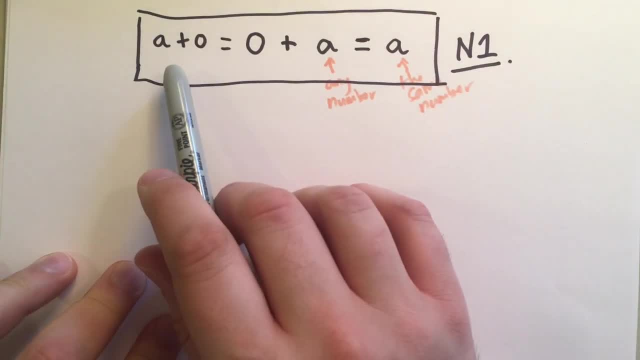 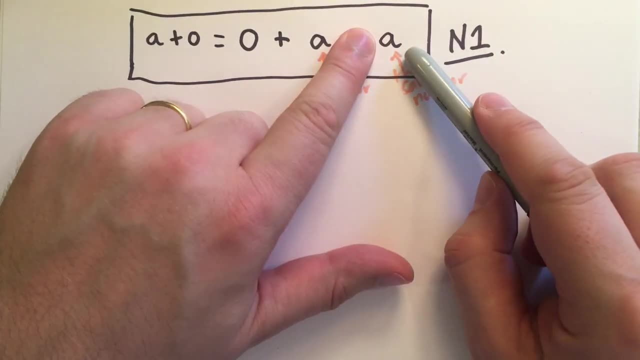 going to talk about n1, the equation n1.. This is the equation we're meaning. When you add 0 to any number, it doesn't change it. Now remember, the equal sign works in reverse. So if you're starting with a, then you can put a 0 on the left side of that or a 0 on that right side and add it together. 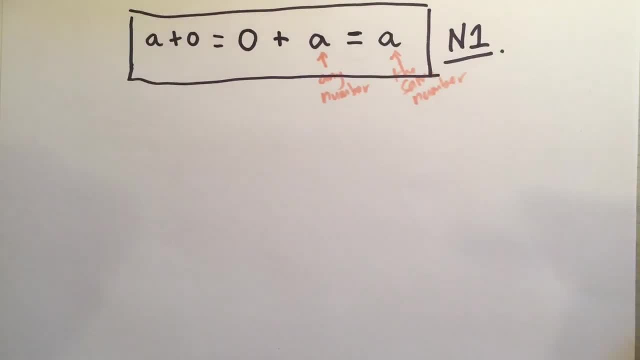 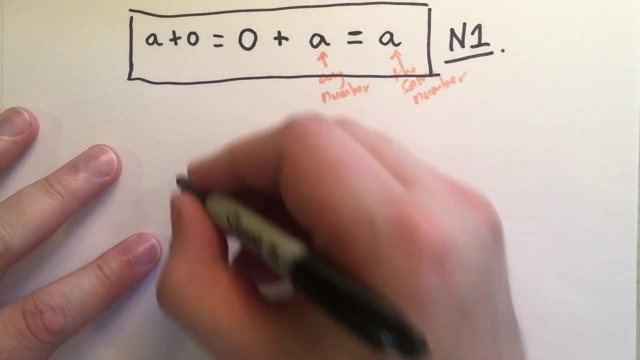 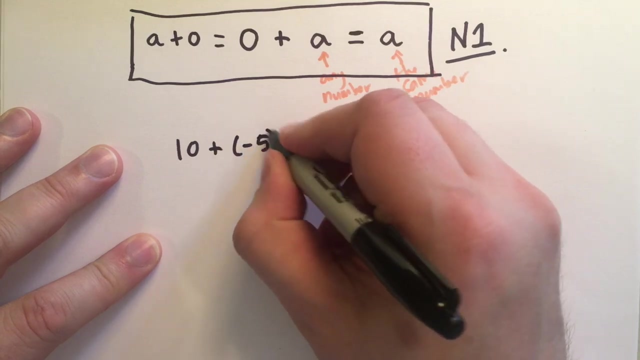 and you won't change the value of a. It won't change how many numbers you have. The next question that you're probably having is what happens when you add negative numbers? What does it mean to start at, let's say, 10 and add negative 5? What does that do? What does that mean? right? 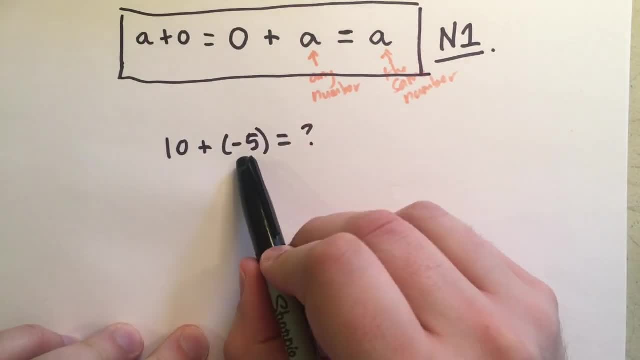 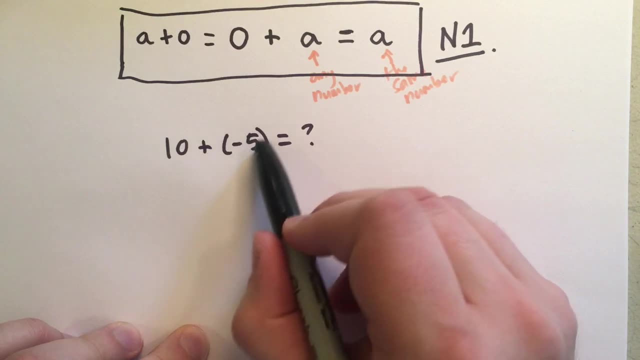 The parentheses here. don't get confused. The parentheses just means we're going to do what's ever on the inside first and then we're going to do what's on the outside later, okay, So this means that we're going to. this is just saying that minus sign there is. 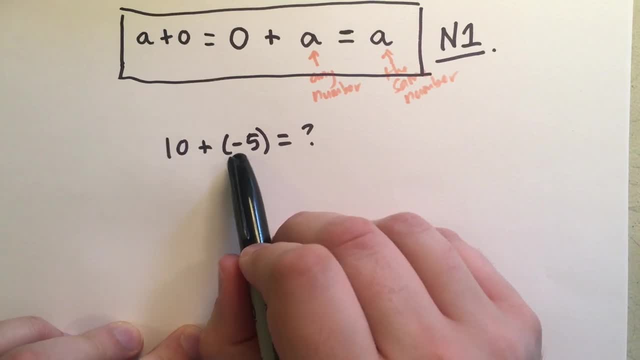 is saying that we're going to do what's ever on the inside first, and then we're going to do what's ever on the inside. So this is saying that this 5 is not a positive 5,, it's a negative 5, but this 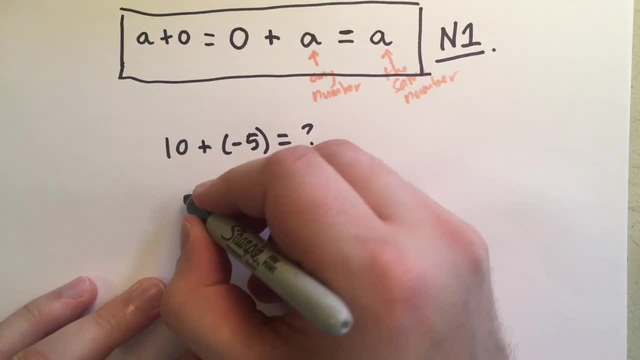 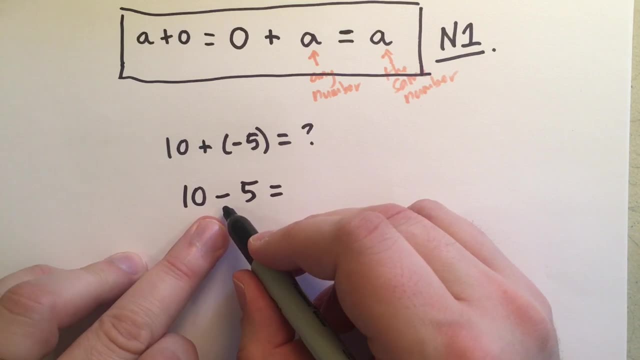 isn't the minus sign you're used to, But let's, let's talk about the minus sign really quick. So, if we have 10 minus 5, what does that equal? Well, that means we're starting at 10 and we're taking. 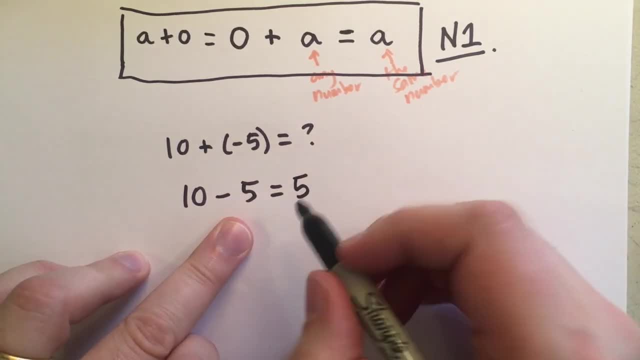 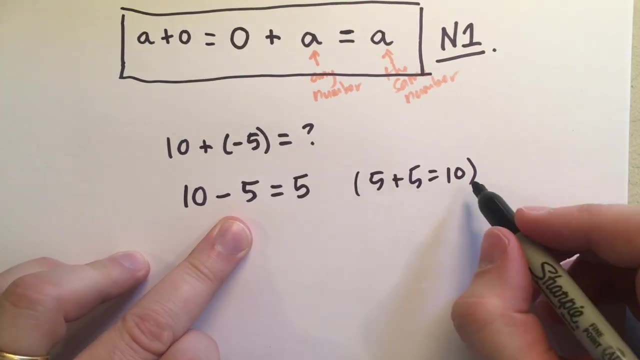 away 5 things. Well, how many would you have left? You'd have 5 left, right, Because- and the proof of this is that 5 plus 5 equals 10, right? We know that 5 plus 5 equals 10, so if we take away 5, 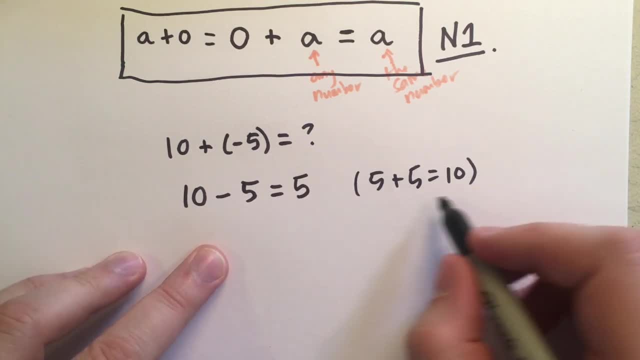 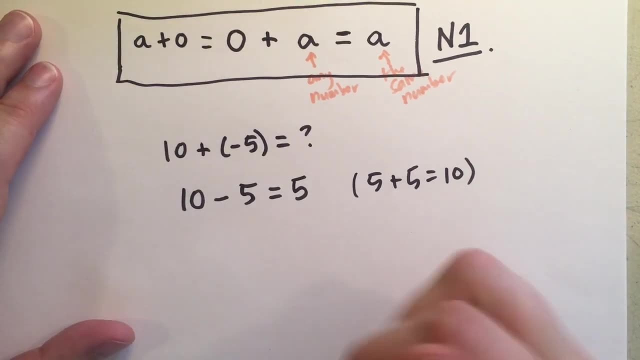 from 10, then we have 5 left over, So this sentence is is related to that sentence in a way that we're going to explore, maybe in the next video, I don't know. Okay, so what happens if we did this, though, If we started at 10 and we subtracted 15,? 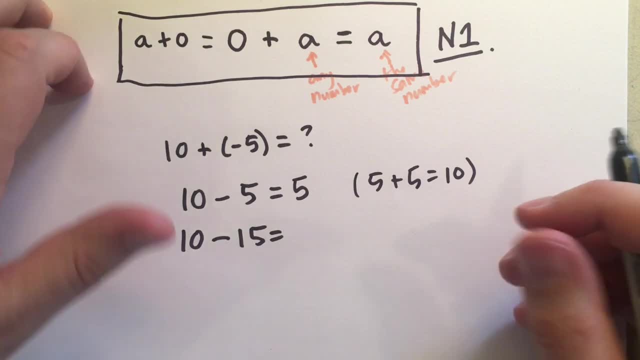 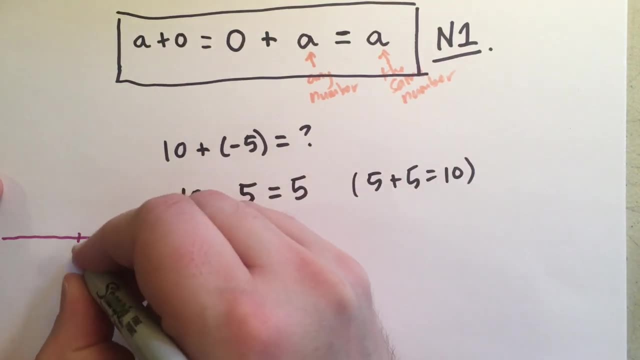 what would we get? That's an interesting question. Let's draw the number line over here. We're going to draw it with a new origin. We're going to put the origin. let's say here: So we have 1,, 2,, 3,, 4,, 5,, 6,, 7,, 8,, 9,, 10.. 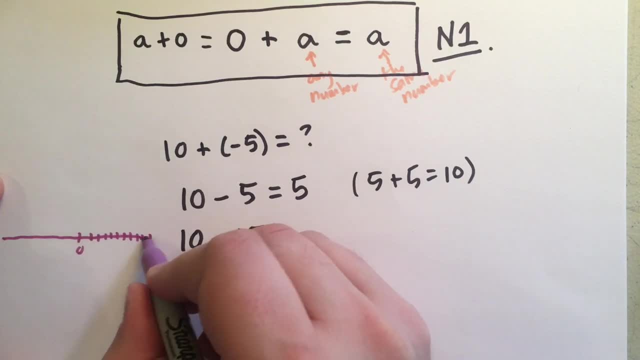 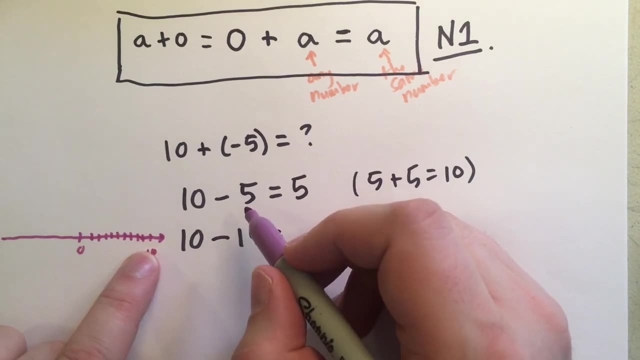 And the 10 here means that you go 10 to the right. This number line goes on for infinity, of course. So we're at 10 to the right. What does it mean to subtract 5?? Well, if you subtract 5,. 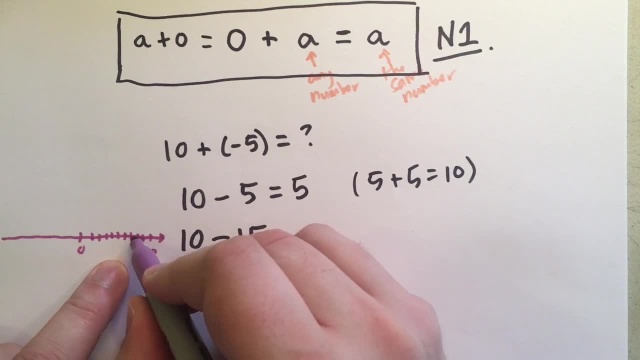 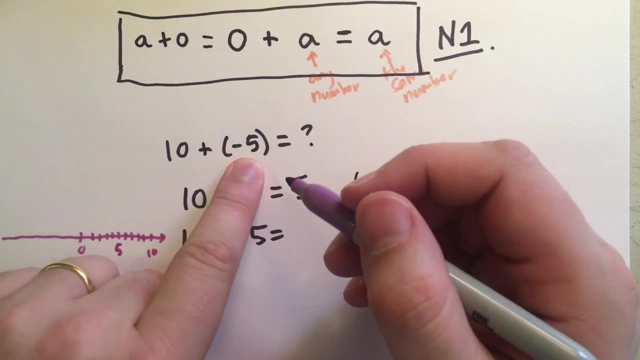 you go back 5 units, So you have 10,, 9,, 8,, 7,, 6, 5.. You can see there's 1 space, 2 space, 3 space, 4 space, 5 spaces. So subtracting or adding the negative means you're moving to. 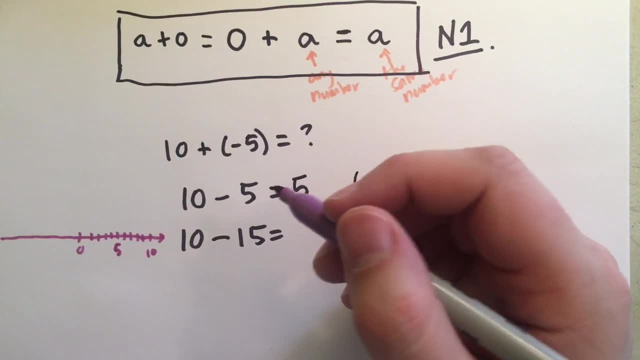 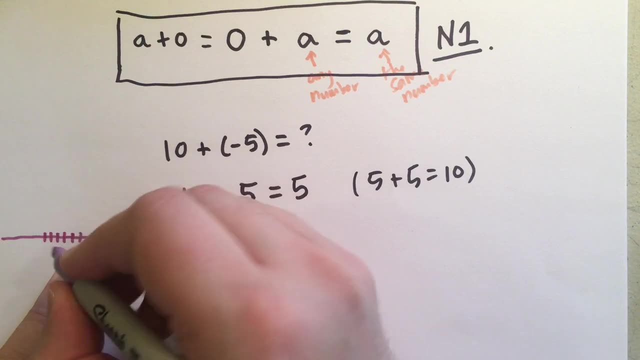 the right. So subtracting or adding the negative means you're moving to the right. So subtracting or the left Adding means you're moving to the right. Okay, So let's move to the left 15 units. So we move 10 units, We're back at the origin: 11,, 12,, 13,, 14, 15.. Well, that's minus 1,, minus 2,, minus 3,. 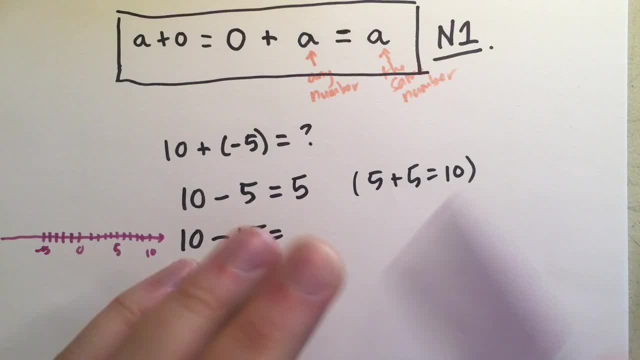 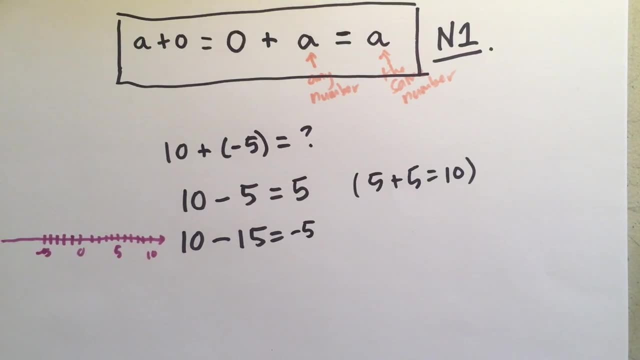 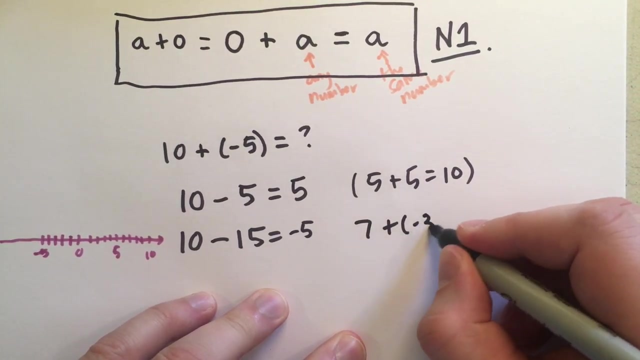 minus 4.. That's minus 5.. So the answer- 10 minus 15, is negative 5.. Okay, That doesn't sound very complicated, does it? Let's do a couple others as examples. So if we had 7 and we added negative, 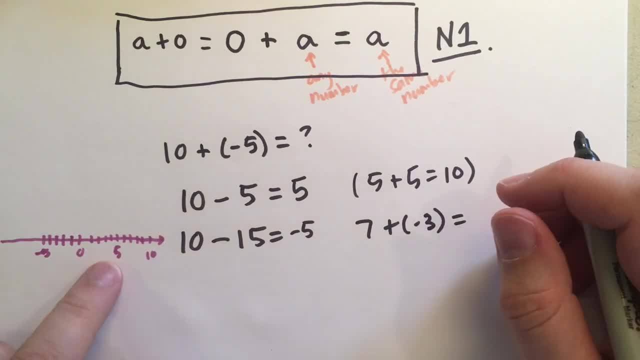 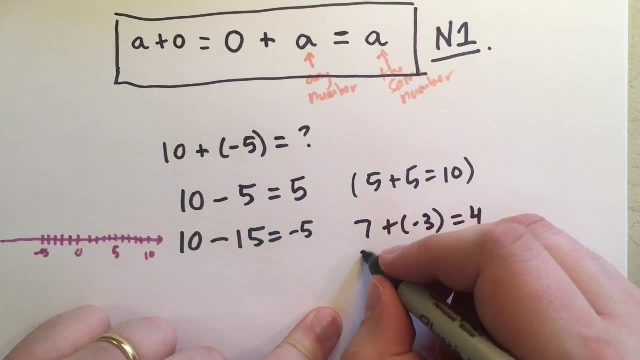 3,. then we would get what? So we start at 7,, 5,, 6,, 7, and go back 3.. 1,, 2,, 3.. We'd end up at 4.. Right, Let's do another one. These are in the book. I'm just duplicating what's in the book. 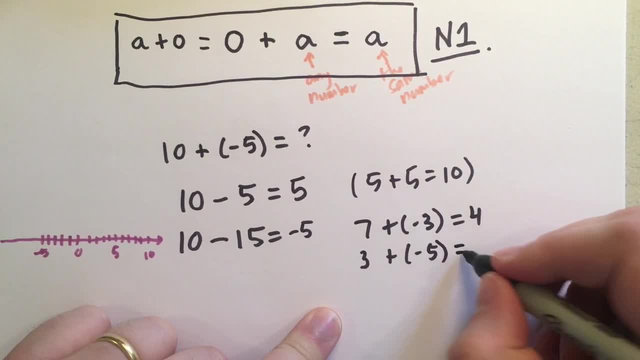 so I don't ruin your study, You should go back and review the books. What if we start at 3?? So 1,, 2,, 3, and we go back 5.. 1,, 2, 3 gets us back to 0.. 4, 5 takes us to negative 2.. Okay, 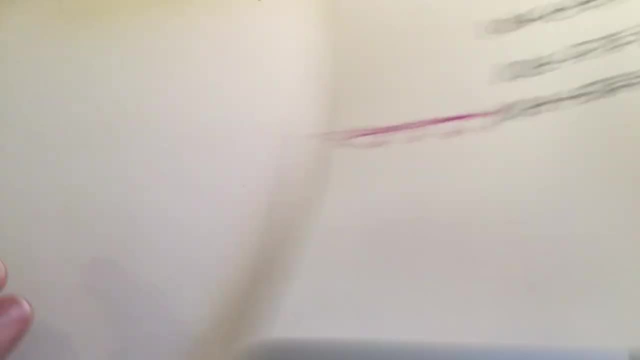 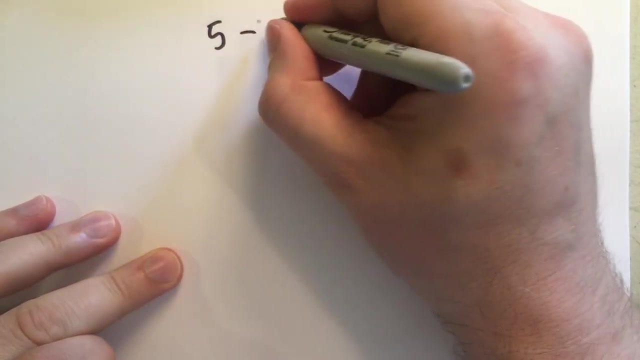 Here's another interesting property. Let's go to a new page, Talk about this property. If we start at 5, slide that down so you can see, and then we subtract 5, that's the same as starting at 5 and adding a negative 5.. And what? 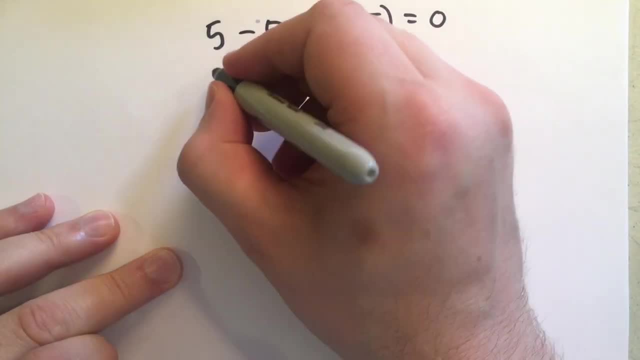 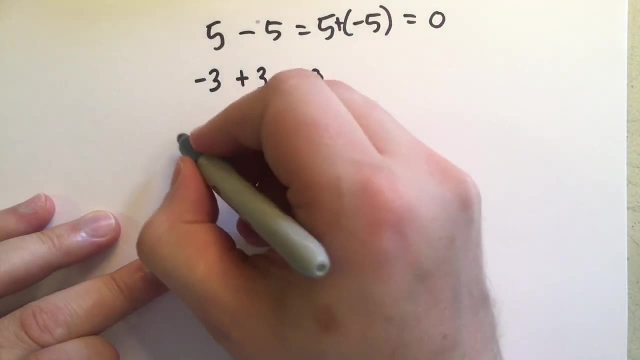 does that give us? It gives us 0.. What if we started at negative 3 and we went 3 to the right? Where does that get us 0.. This tells us that when we start with any number and we add its. 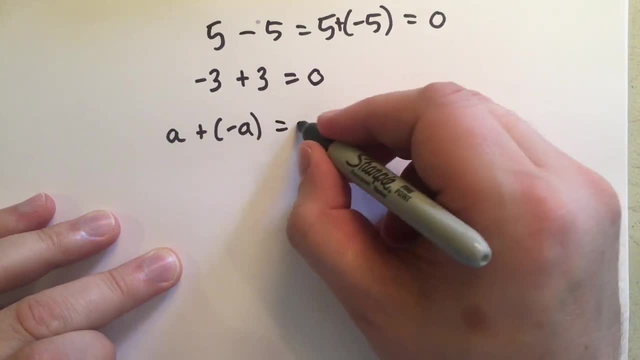 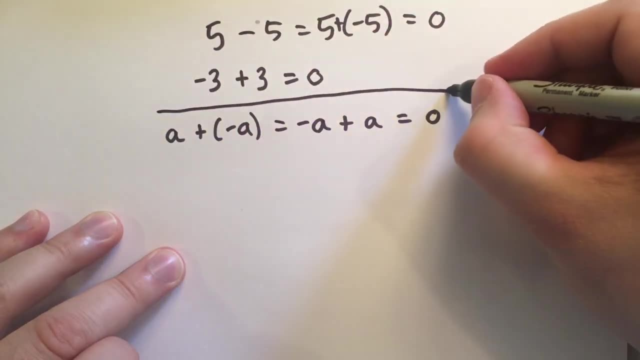 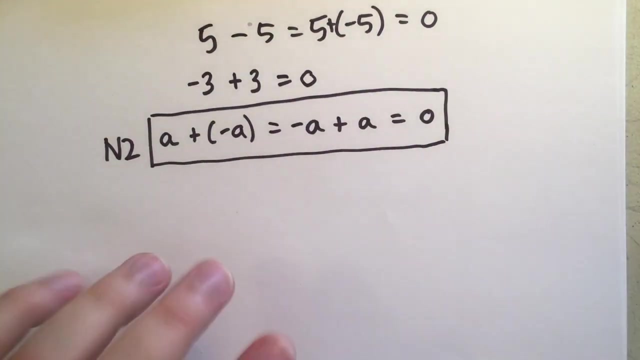 negative counterpart. it's the same as starting at the negative counterpart and adding that same number. It's the same as 0. This is equation N2.. And this is a very important property that we use all the time when we do math. So, just like in N1, we discovered that we can add 0 to any number. 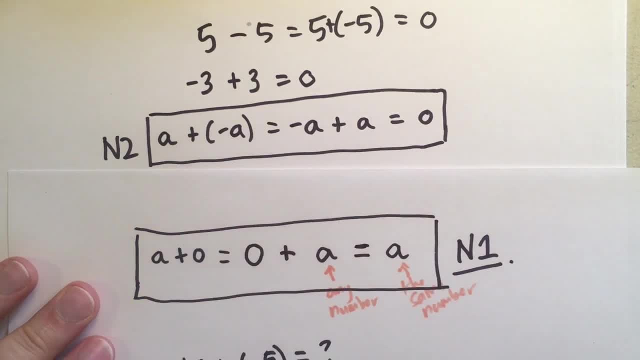 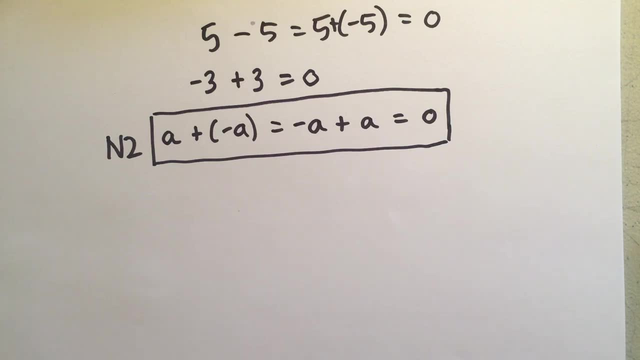 In N2, we discovered that we can get to 0 from any number, positive or negative, by adding the inverse additive- inverse, what we can call it- On the number line. what does this look like? Pull out my little pink. We have the number line here. It goes off to the right, It goes off to. 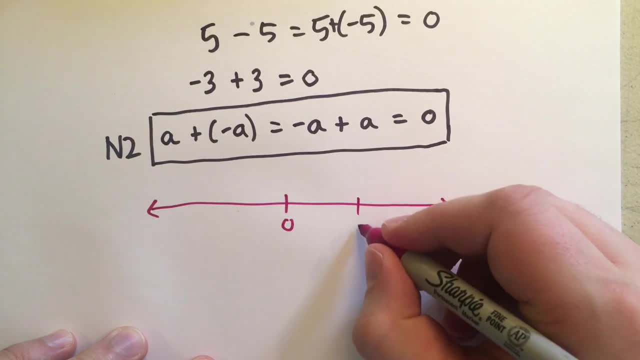 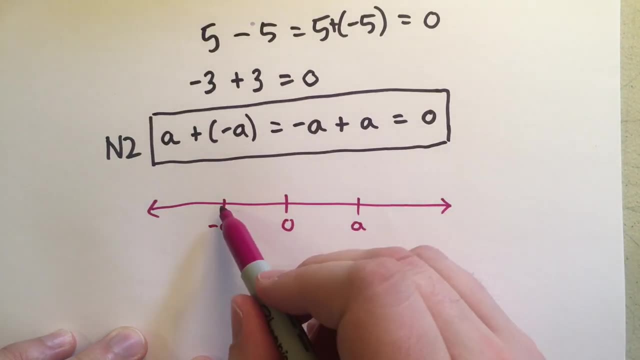 the left. Let's put zero in the middle this time. If we start at A and we go back negative A steps, we get back to zero. And if we start at negative A and we go forward A steps, we get back to zero. 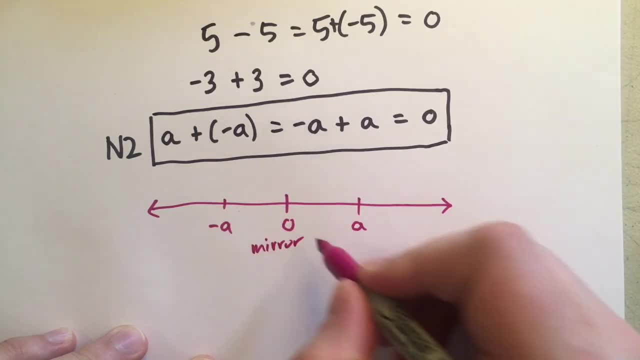 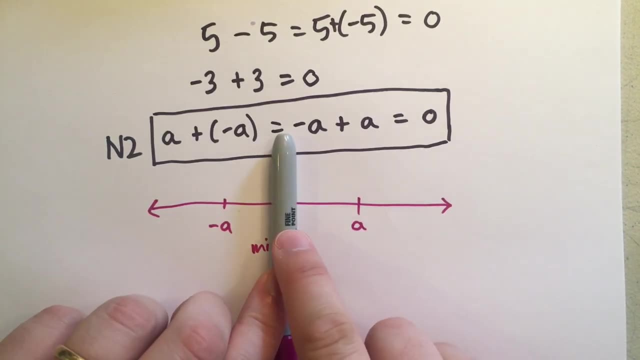 This is sort of a mirror, with the origin being the plane of the mirror. So the reflection: when A looks in the mirror, it sees negative A, And when negative A looks in the mirror, it sees A. So the positive and the negative realms are sort of mirror images of each other. One goes 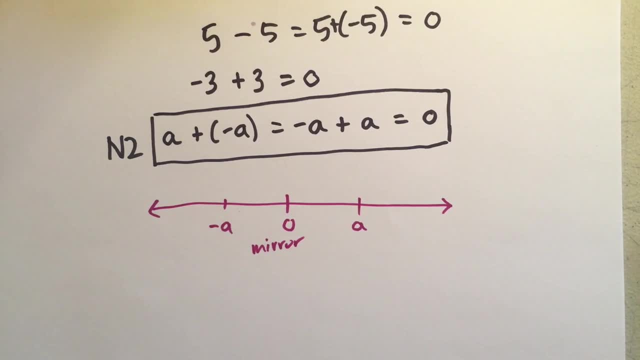 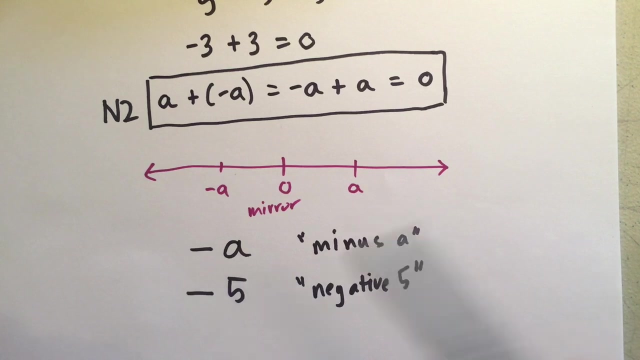 to the right while one goes to the left. All right, Note, and this is important: we say minus A And we say negative five. Okay, What is the difference? Well, the difference is what, if A was, if A was, let's say, negative three, then minus A would be three. Minus A is not negative. 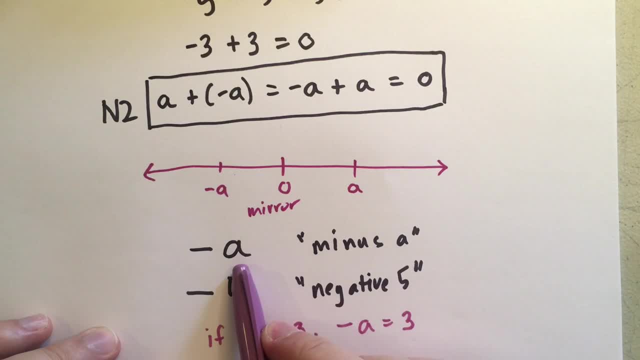 It's positive. So if you don't know that A positive you you can't say that this number is negative. you have to say it's minus a. it's important distinction. you'll often hear people when they're doing their math lectures they'll say negative a when it's not really negative.